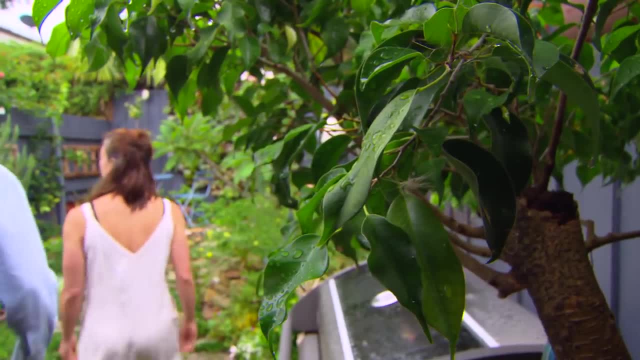 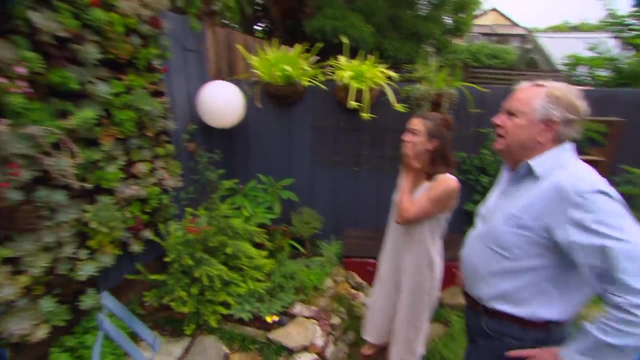 thing that we might inherit from the house when we arrived. Come into my world. I've got to show, show, show you, And will you look at this? What a great green wall. that is My pride at the moment. How many years old is it? 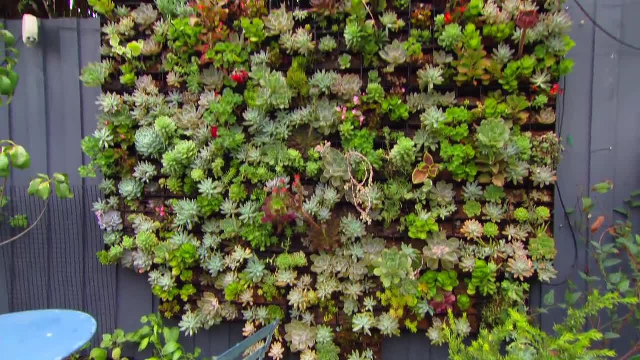 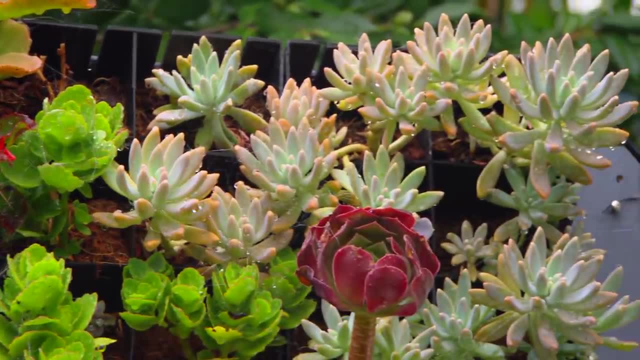 I put it up there about a year ago. You've got a really interesting collection of plants. Where did you buy them all? Well, my mum gave me most of the succulents on the wall and they grow actually fairly quickly, so I just chop them up and put them in new cabinets. 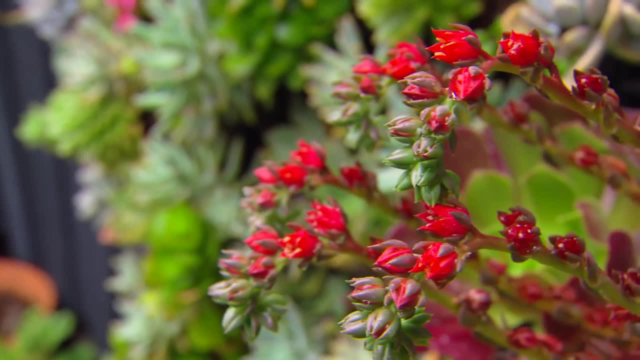 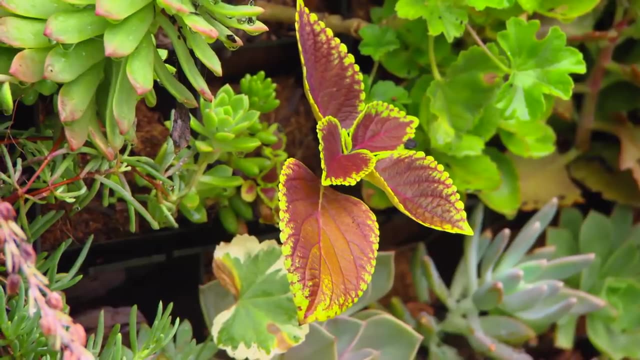 And they just keep multiplying. You've got a bit of a big red in there as well. I've got a big red in there. It's uranium, And begonias- The begonias And acolias, Yes. Now if you prune them back and then spray a bit of fertiliser on them, they'll come back- Awesome. So you've got the permanent root system. Yeah. 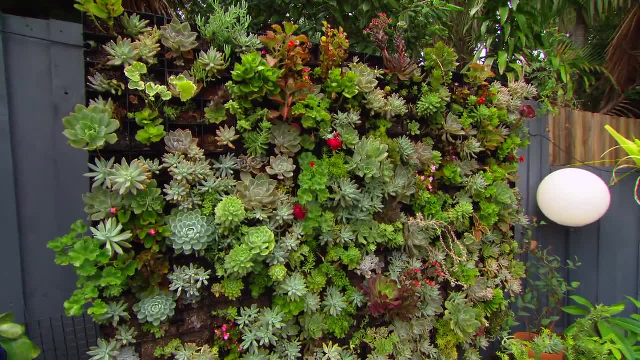 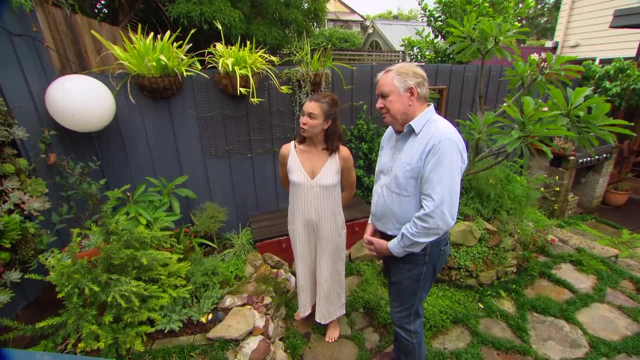 And then new, fresh growth, because it gets a little bit ratty after a while when they finish flowering. Okay, The other problem that a lot of people ask me about is potting mix. So how did you overcome that problem? I tried a few different things and I've kind of settled with it. 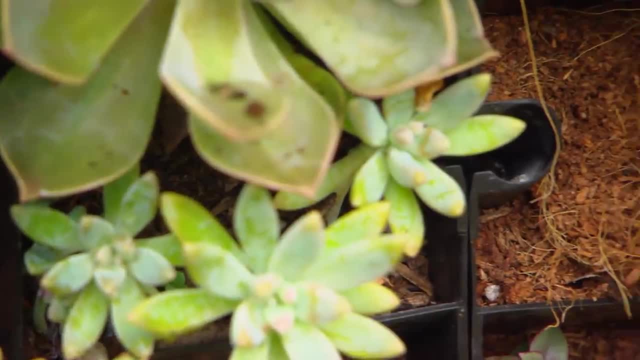 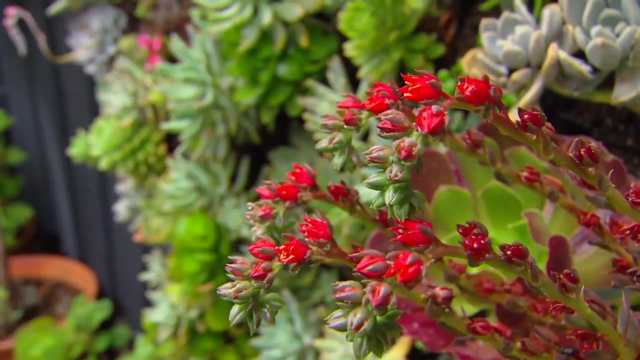 I've got some coir, Oh, coir, Pete. Yeah, Pete, Shove a few water crystals in just to help them. One of its advantages: coconut fibre. it'll stay where you put it. Yes, it doesn't fall out. That's really clever. 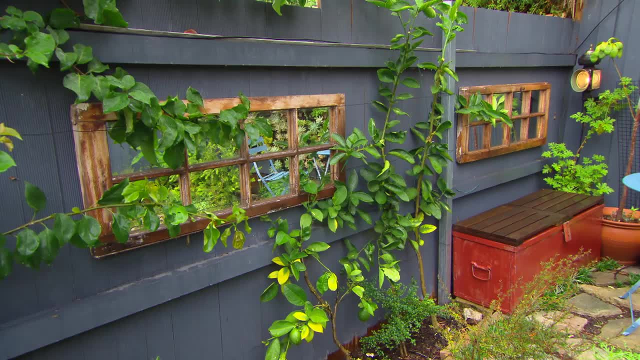 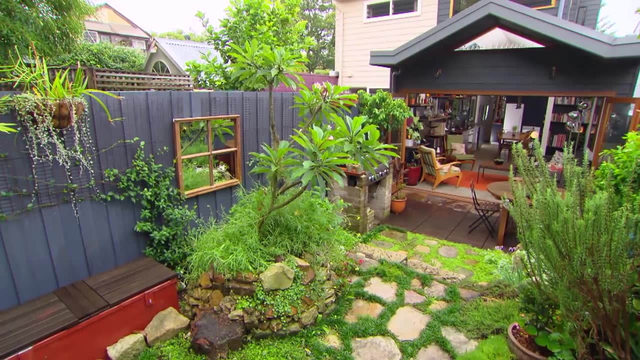 The couple have used some very smart ideas to make the most of such a small area. There's no actual boundary between the house and the garden. It comes right out into the landscape, And the grey that was inside the kitchen is now the fence colour. 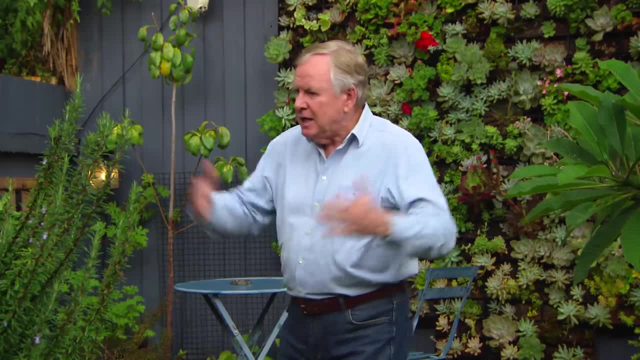 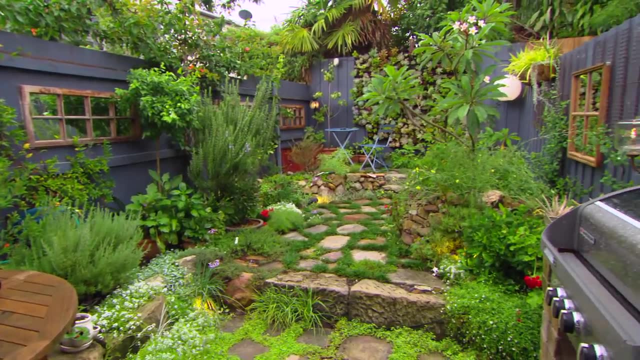 Have a look what they've done here. Some very clever little tricks. Firstly, the verticals. That's what you've got to look at. They've created a lot of privacy here. They've got some wire on both sides that they're growing. star jasmine, some gel semium, the Carolina jasmine. 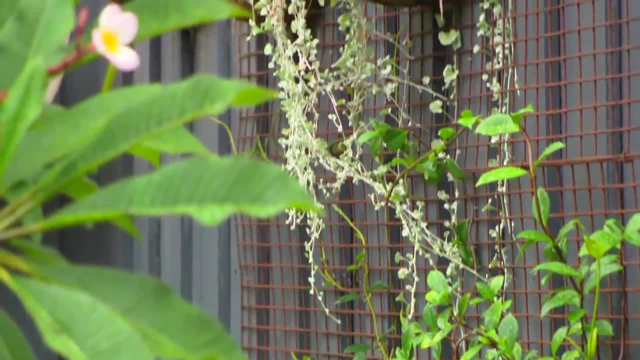 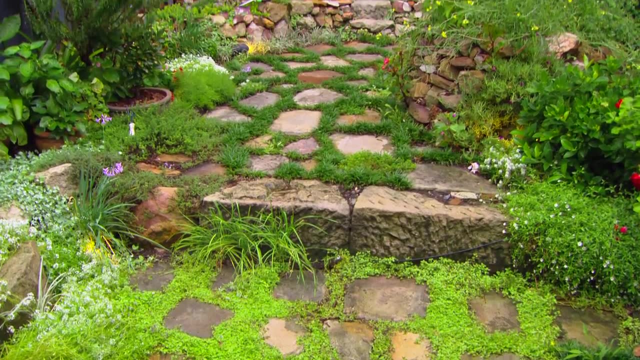 And then, of course, you've got the hanging baskets of the creeping iris up there And, of course, once you've solved the verticals, it's then the horizontal Look. you go from one level to the next, to another level, right up the top here. 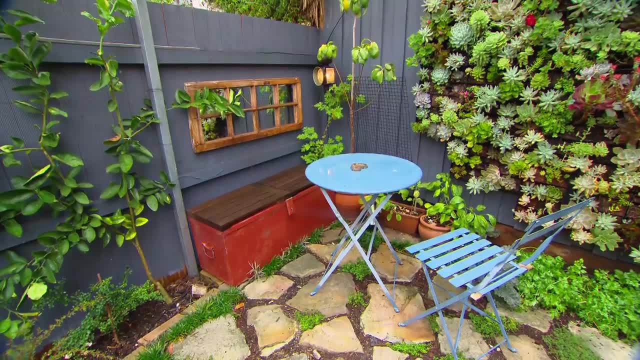 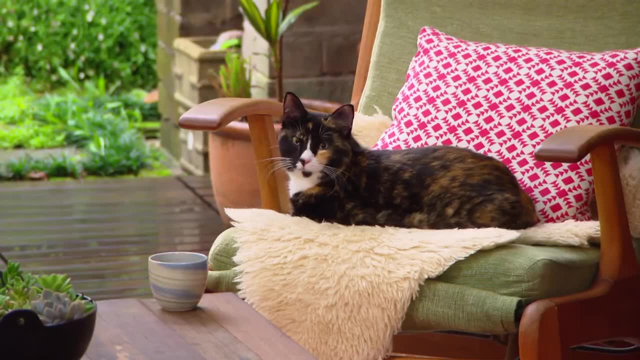 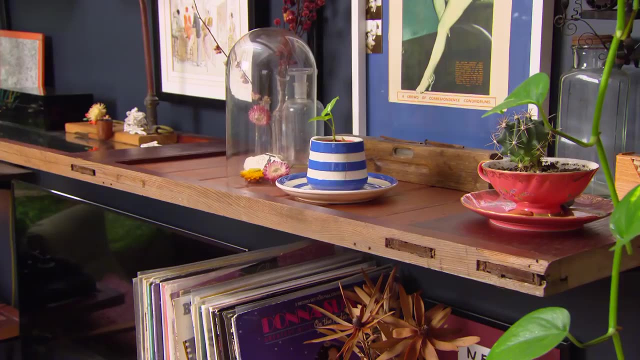 And that all creates interest, And that all creates interest in a very small area. It's only a small garden, but it feels like a very big space, Not only great out in the garden, but you've built most of this yourselves inside.